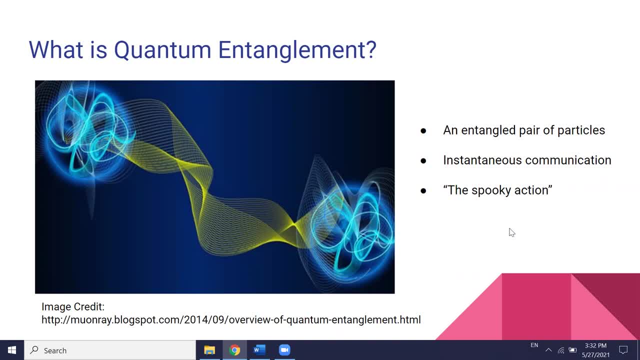 with exact perception, For example, such as the famous Heisenberg's uncertainty principle, implies a limit to the accuracy of a simultaneous measurement of the position and the momentum variable pairs. On the contrary, quantum entanglement describes the two components of a quantum system connected with one another in such 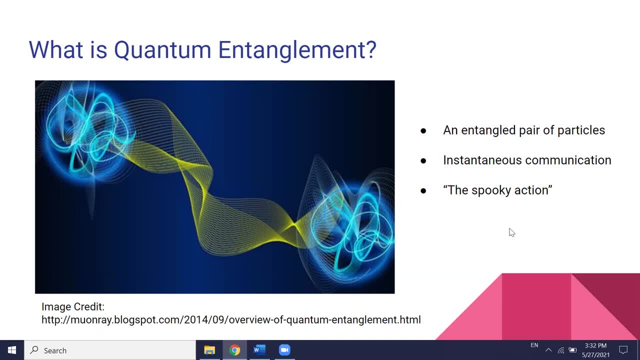 a way that the quantum status of each component cannot be described independently, even if the pair of the components say there are, particles are separated by a large distance. For instance, if a pair of photons initially interact, no matter how far away they are. 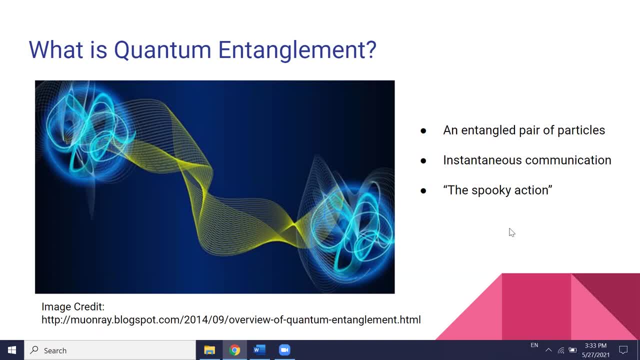 separated. later on, when an observer measures the state of one photon, the other photon state will be instantaneously determined For spin-1 half particles, spin-2 half particles. if one particle in the entangled pair is measured to be spin-up state, the other one 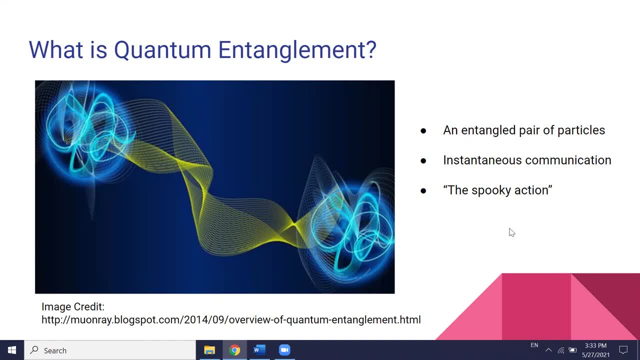 may be instantaneously forced to be in the spin-down state. The reason is because the initial interaction or the entanglement between those two photons allow them to be defined by a single wave function. Once they are separated later, they will still share the same wave. 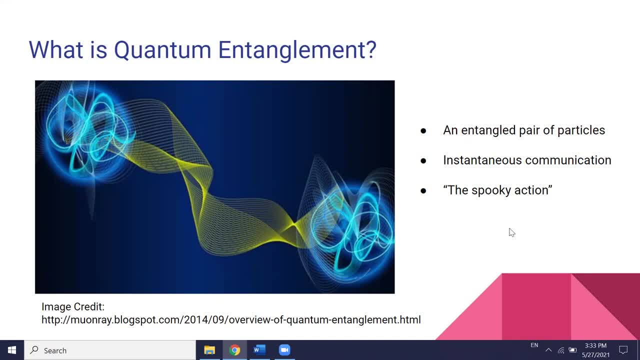 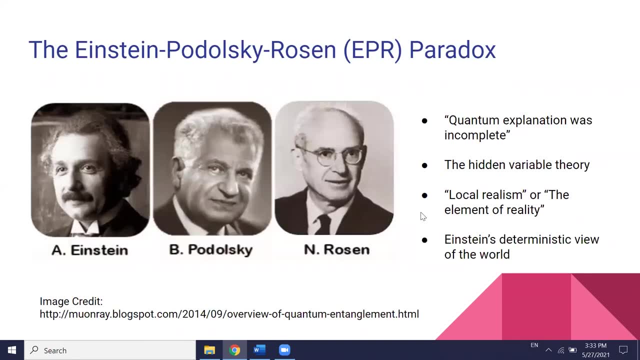 function. Einstein described the quantum entanglement as the spooky action due to the strange behavior. In 1935, three physicists- Einstein, Podavsky and Rosen- published a paper titled Can Quantum Mechanical Description of Physical Reliability be Considered Complete and introduced a thought. 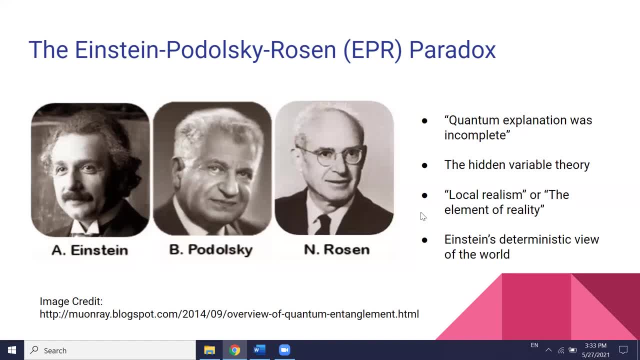 experiment to argue that a quantum explanation of entanglement was an incomplete theory. Based on quantum entanglement theory, it is said that the result of a measurement of one particle of entangled pair systems can have an instantaneous effect on another particle, regardless of the distance between the two particles. 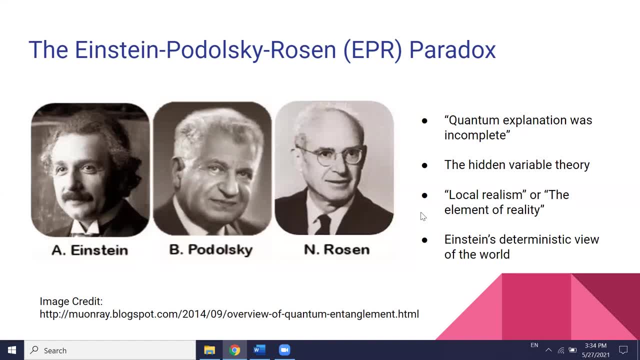 The EPR paradox suggests that the equation of the two quantum particles is a proof of described quote. either the quantum mechanical description of the reliability given by a wave function is not complete, or when the operators corresponding to two physical quantities do not commute, the two quantities cannot have the simultaneous reliability. Therefore, the EPR 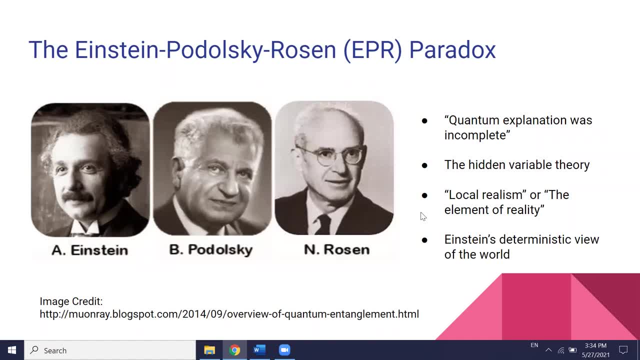 paradox, considers quantum theory as an incomplete theory. It is important to notice that Einstein and his colleagues were not against the quantum theory, but to demonstrate the innate conceptual difficulties of the quantum theory. So to the question: can quantum mechanical description of physical reliability be considered complete? Einstein's answer was clearly negative. As a 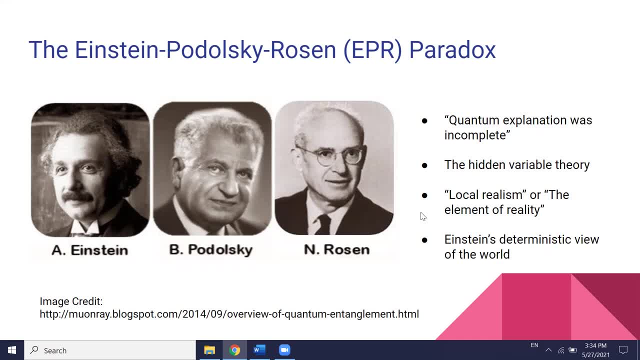 solution to the paradox. Einstein postulated the existence of the hidden variables- as yet unknown. hidden, as yet unknown local properties of the system which could account for the disparity, sorry discrepancy, so that no instantaneous spooky action would be necessary. This is known as the 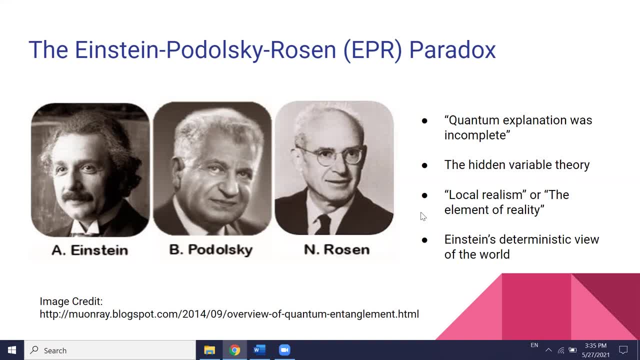 local realism or element of reliability which reflects Einstein's deterministic view of the world. EPR paradox described the principle of locality as asserting that physical processes occurring at one place should have no immediate effect on the elements of reliability at another location. The implication of the EPR paper. 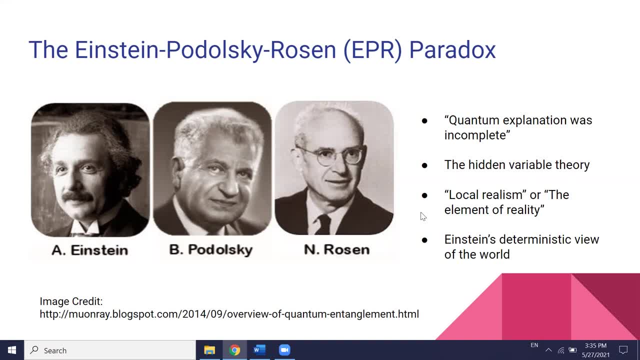 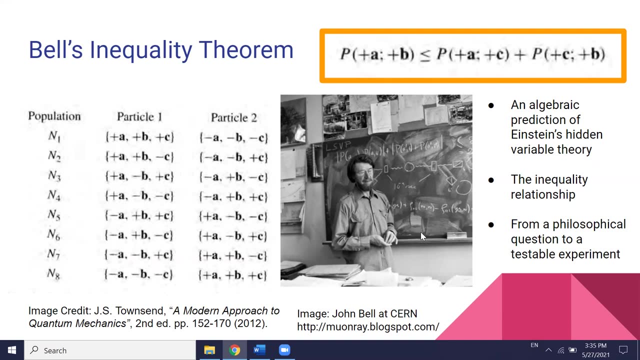 for instance, is to illustrate how quantum physics is not the same as classical physics, which helps deeper our understanding of non-classical characteristics of the quantum world. So in 1964, a physicist named John Bale published a paper titled on the Einstein-Podolsky-Rosen. 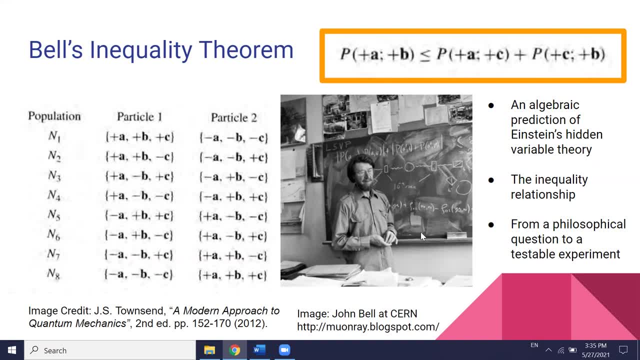 paradox. as a response to the EPR paradox, He pointed out an alternative theory based on the EPR's locality principle that actually yields a testable inequality that differs from predictions of quantum mechanics. Bale proved that Einstein's point of view, or local realism, 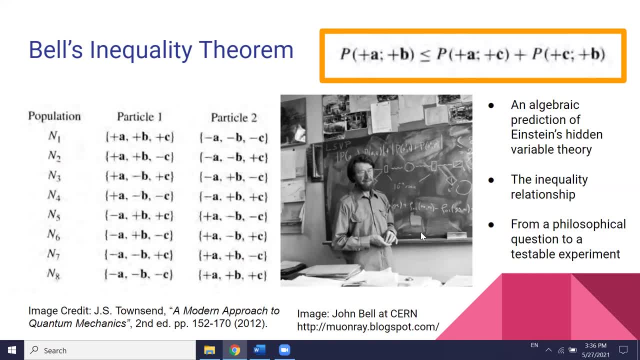 leads to algebraic predictions. His work translated Einstein's philosophical position of the realism and locality into a precise mathematical description In the Sting-Gerlach experiments. let's consider an experiment in which A and B orange their S-G-veis at random along the 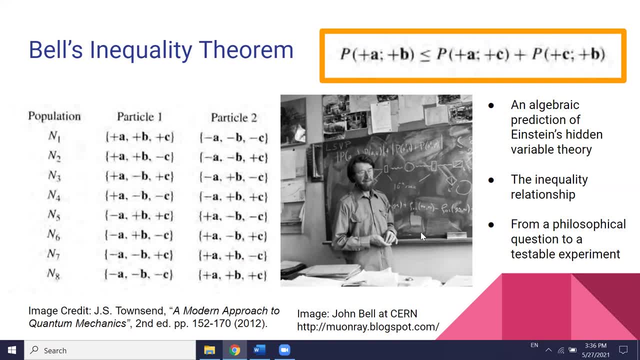 axis A, B and C, making measurements of the spin of particles along this axis In order to conserve the angular momentum, for instance when theVisor is satellites. the coordinates of the first two angles are based on the simultaneous range of. with respect to the rate of evolution, The 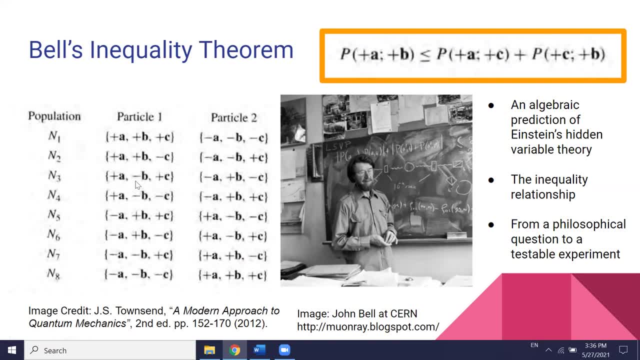 For instance, if particle 1 is in the type, then particle 2 must have the type, so that if A finds particle 1 to have a spin up or down along the same axis, B finds particle 2 to have a spin oppositely directed along the same axis. 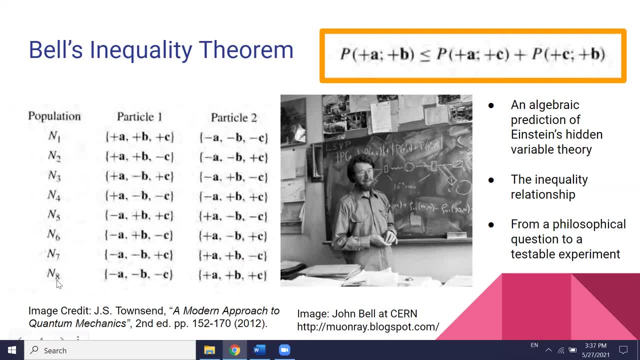 As a result, there are in total eight combinations that the two particles can emit in the decay of a spin-0 particle, which is shown in this chart here. So to match the result of the Stinger lock experiment, we will find that EPR's hidden variable theory must satisfy this inequality equation in this orange box. 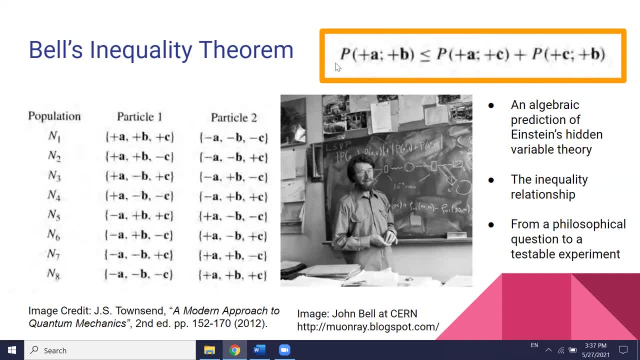 So, in order to test this inequality, A and B must make measurements to determine the three probabilities. First, A's S-geo device is oriented along A, while B's fix along the B axis, and the measurements are made to determine the probability of plus A, plus B. 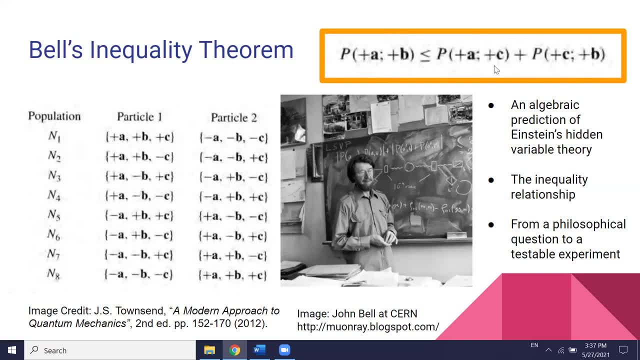 A and B. then go to measure the probability of plus A plus C and plus C plus B to see if the inequality is satisfied. So the inequality is in the form that is easy to compare: the predictions of the quantum mechanics: If quantum mechanics is correct and the Bills inequality is correct. 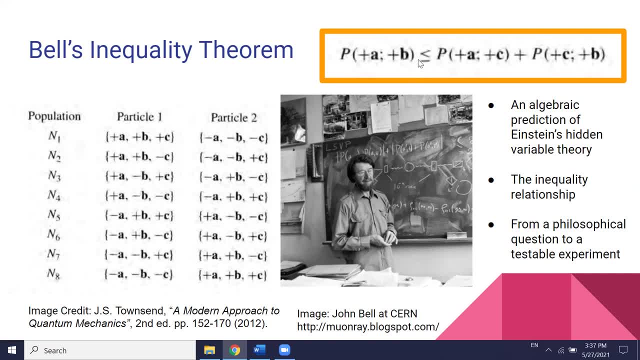 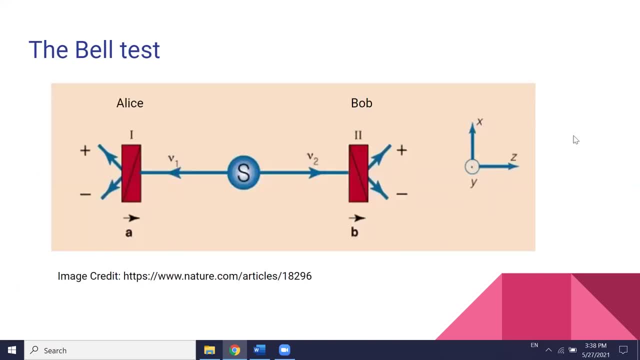 then EPR's hidden variable theory must satisfy the equation in this orange box violated, No local hidden variable theory can be valid. Now let me introduce you to the idea behind the Bill test, as well as some interesting experimental results that test Bill's inequality theorem. 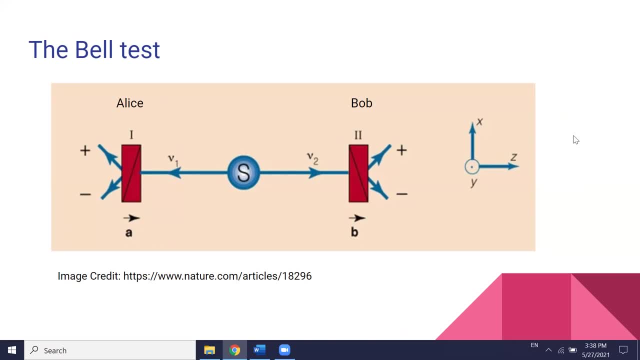 So recall that Bill proved that the quantum mechanics is incompatible with Einstein's local realism. right, Bill? tests are experiments that are designed to test whether or not the real world satisfies the local realism. An experimental can produce a pair of entangled particles and send them to two separate measurement stations. 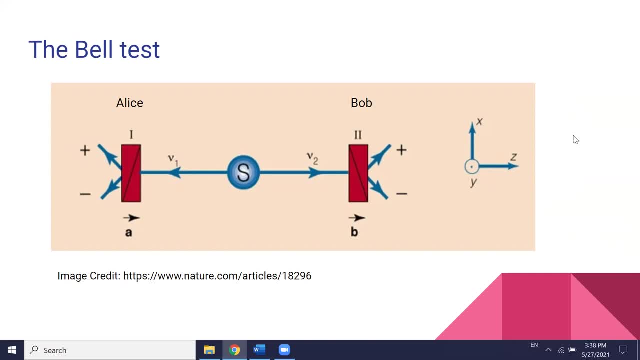 To observers. Alice and Bob stay at each station. Alice and Bob are in charge of making simultaneous, unpredictable measurements on each particle. Quantum mechanics predicts that the measurements Alice makes will instantaneously influence Bob's particle and vice versa, Whereas the local realism predicts that 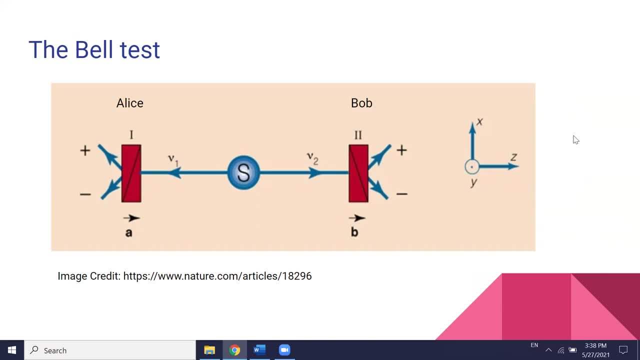 this isn't possible. influence cannot happen and Addis and Bob's measurements should not agree with each other. Following the idea that Bill's inequality is testable, many scientists have designed different kinds of experiments to test whether Einstein's hidden variable theory or the quantum world is. 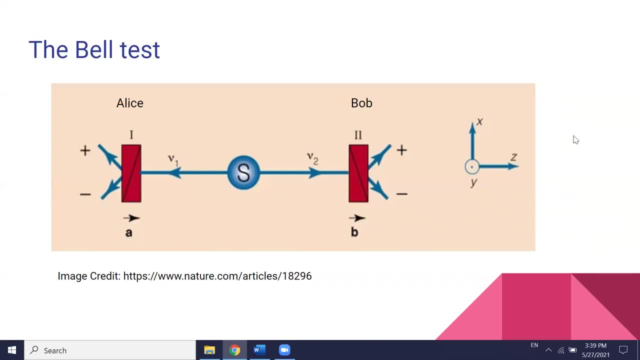 correct. Many types of Bill tests have been performed in the physical laboratories since 1970s. People are constantly designing better experiments to close the so-called loopholes that may cause the flows or the errors of experiments. Such loopholes may be from the. 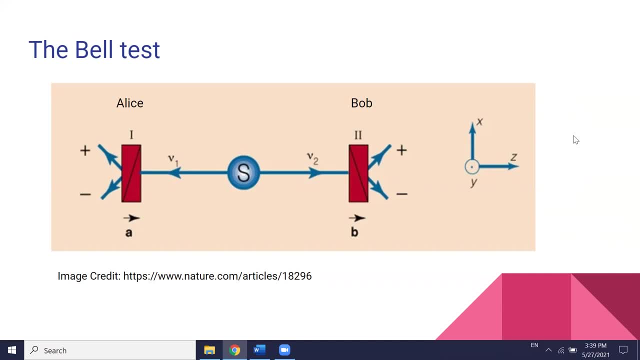 design or the setup of experiments, or if the observers indeed have the free will to ensure the unpredictability of Bill tests. The freedom of choice loophole refers to the idea that experimenters have total freedom in choosing their experimental sets from the types of particles. 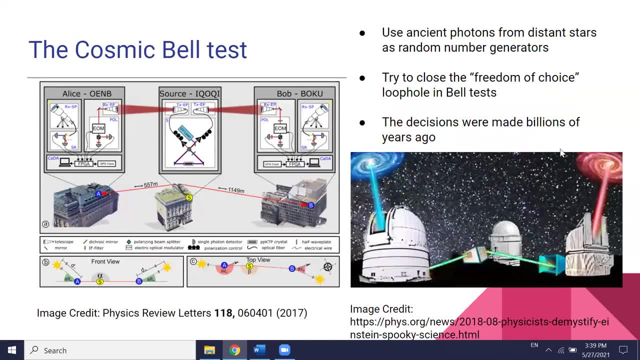 to the measurements they choose. One of the most famous experiments is the one that I just showed you. It's the cosmic Bill test In 2014,. scientists proposed experiments using the Asian photon from astronomical sources such as stars as random number generators rather than the generators. 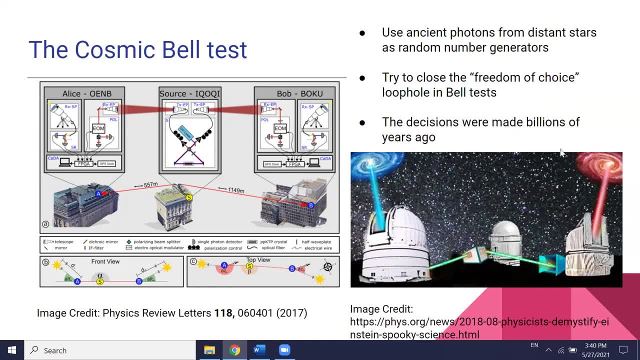 on Earth. Here the left picture shows you that researchers set up the telescope at three detector stations and detect the photons from the stars. The stars are anywhere from dozens to billions of light-years away from the Earth. Thus, if some hidden variable theory is not, 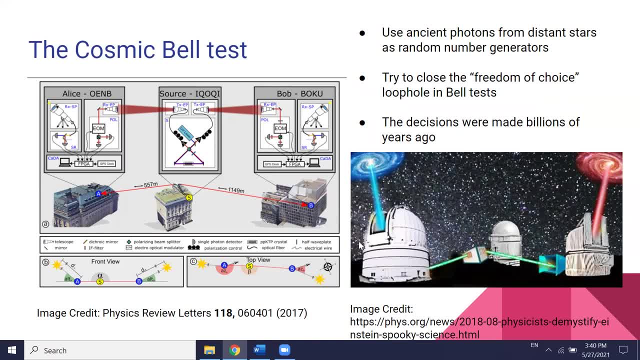 true, they would have to set those up before the time that light left the cosmic sources and reached Earth, which is impossible In a few microseconds before an entangled stellar photon arrived at the detector, the researchers used each telescope to rapidly measure the properties of an incoming stellar photon, to see whether its wavelength was red or blue. 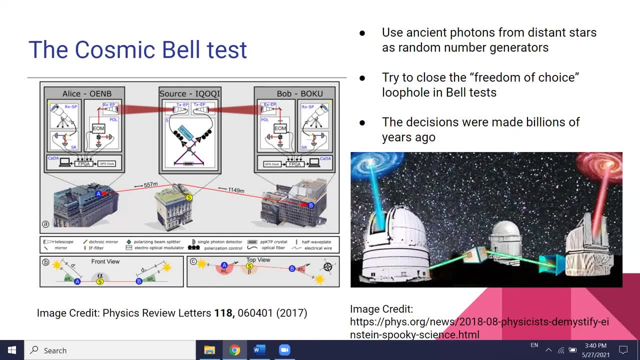 The red photon refers to the detector measuring an entangled photon's polarization in a particular direction, whereas the blue photon measured the polarization of an entangled particle along a different direction. As a result, the researchers measured about 100,000 pairs of entangled 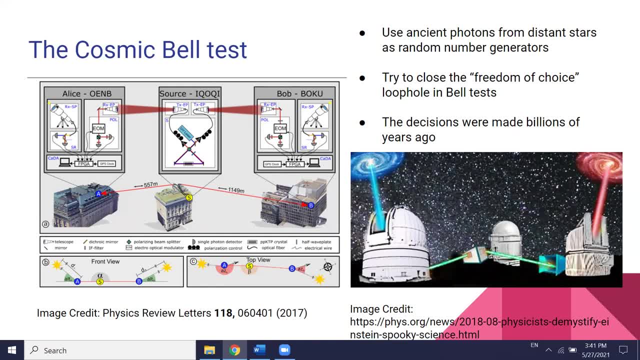 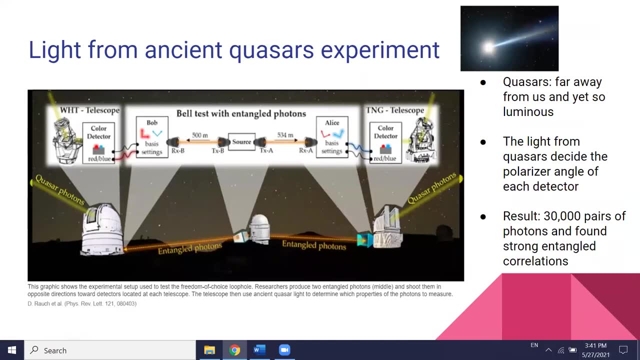 stellar photons and found that the polarization measurements of the photon pairs were highly correlated. This result showed consistency with the quantum entanglement and violated Bill's inequality theory. So, following the cosmic bill test, researchers designed and conducted a similar experiment with much larger and more powerful telescopes to catch the incoming light from even more. 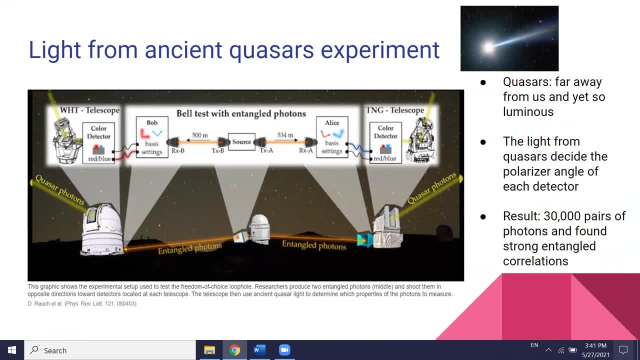 ancient distance astrophysical sources. the quasars, Quasars, are astronomical objects that are incredibly far away and yet are so luminous that light can travel to Earth. In this experiment, researchers used the light from two distant quasars as their random number. 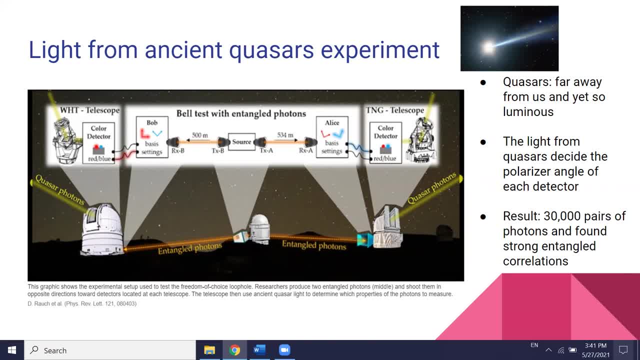 generators, one of which emitted the light from an entangled stellar photon and the other from 12.2 billion years ago. They set a telescope for detecting light from each quasar respectively. The light from quasars decided the measurement choice, the polarizer. 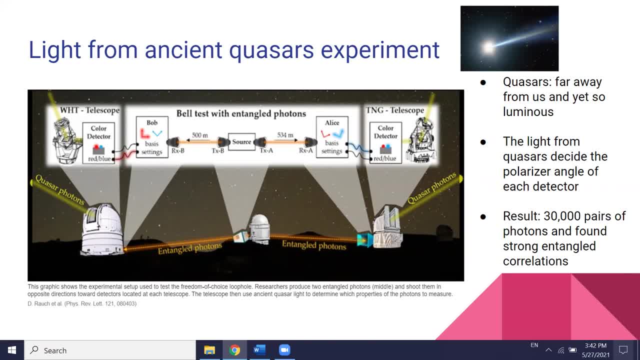 angle at each detector. Meanwhile, researchers at a station located between the two telescopes created pairs of entangled photons based on the measurement choices of two ancient quasars. As a result, they measured more than 30,000 pairs of photons and found strong entangled 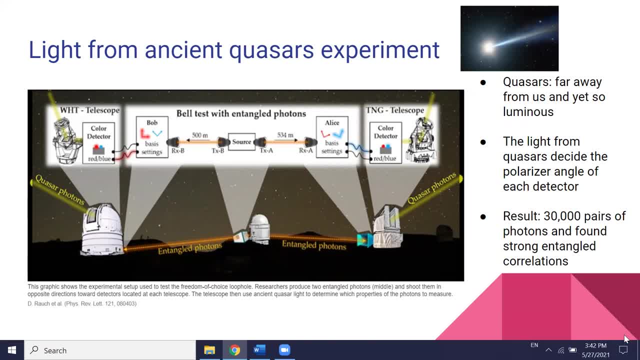 photons among them to a degree that far exceeded the limit of Bill's original calculation predicted. Once again, the hidden variable theory is disapproved by the experimental results. Then I would like to introduce you with another very interesting bill test called the Big. 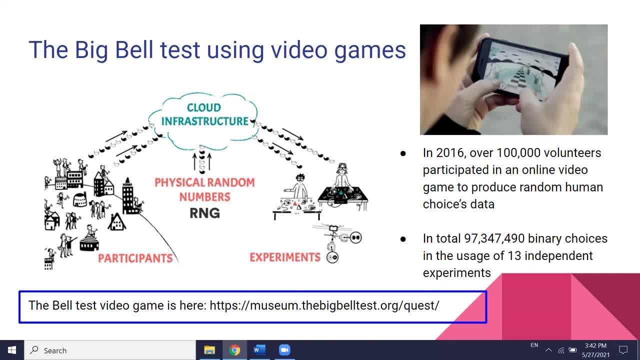 Bill Test in 2016.. The Big Bill Test is a worthwhile project using video games to bring human unpredictability or human randomness to cutting-edge physics experiments. The Big Bill Test is a worthwhile project using video games to bring human randomness to cutting-edge physics experiments. In 2016,, over 100,000 volunteers participated in an 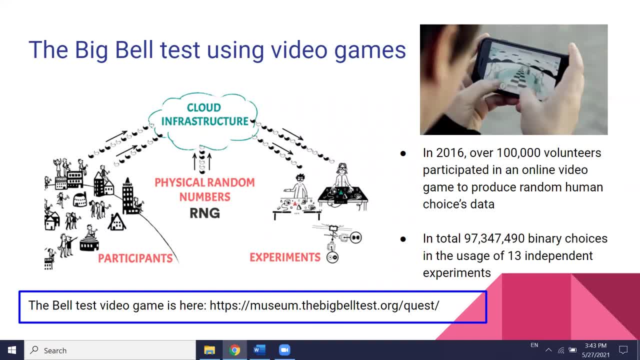 online video game that used random human choices to produce the data for researchers conducting multiple independent tests across the globe On November 30, 2016,. during a 12-hour period, the participants worked well and provided a sustained data flow of over 1,000 bits per 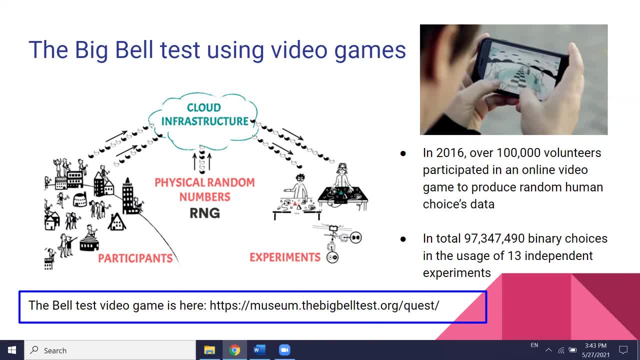 second to a Big Bill Test experiment. The participants generated in total 97,347,490 binary choices in the usage of 13 independent experiments that tested local realism using photons, single atoms, atomic assemblies and superconducting devices. This video game. 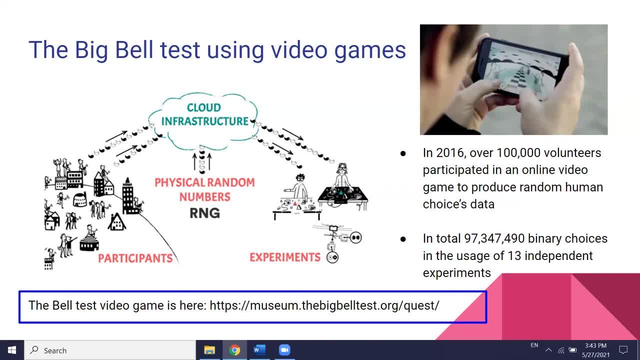 method provided rapid collections of human-generated randomness. As a result, most experiments observed statistically strong violation of their respective inequalities, supporting rejections of local realism in a multitude of systems and scenarios. Until today, there have been many experiments that are followed by the Bill's Inequalities Theorem. Those 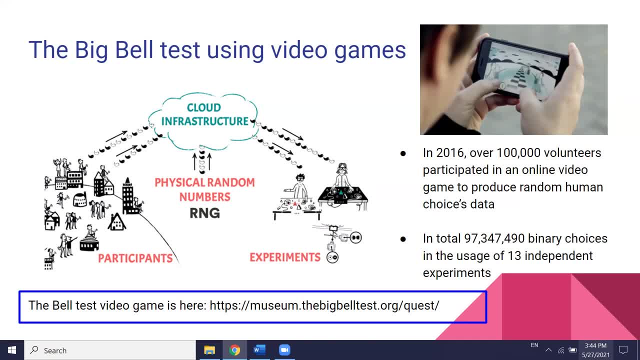 experiments are designed to test whether Einstein's Hidden Variable Theory is correct or not. As for now, all of the experiments have found that a hypothesis of Hidden Variable Theory is inconsistent with the way that the physical universe broadcasts it. This is why the Big consistent with the way that the physical system behave. 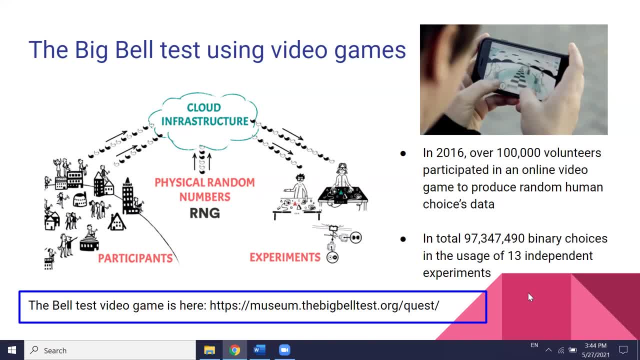 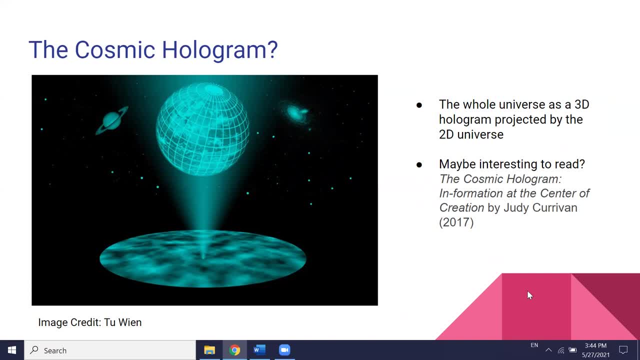 Very likely Einstein was wrong in this case. So you may want to ask a question like: why does the weird quantum entanglement exist? Well, no one actually knows, but scientists have provided many cool hypothesis. One of them is called a cosmic hologram. 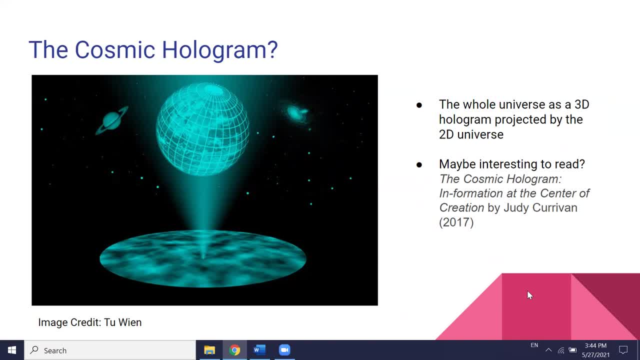 which follows the idea that, since two entangled particles can instantaneously communicate with each other, regardless of the large distance among them they can, then we can probably say that the space between them somehow do not exist. So, following that idea, we're probably living in a 3D holographic world. 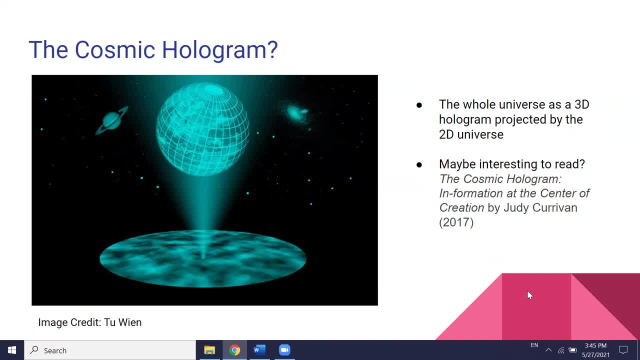 that is projected by the 2D world, like this picture shows you. This idea may sound crazy for you- for me as well- but I find it's kind of intriguing, and here's a book you may want to read and get more knowledge about that. 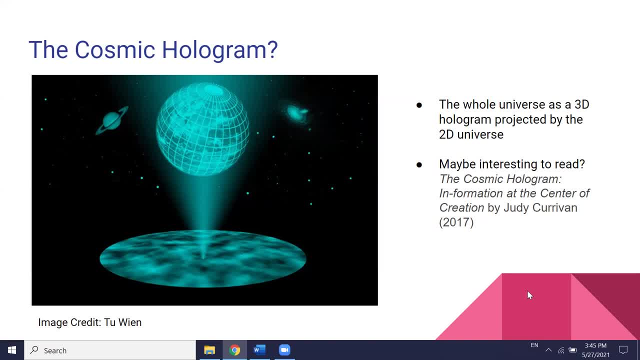 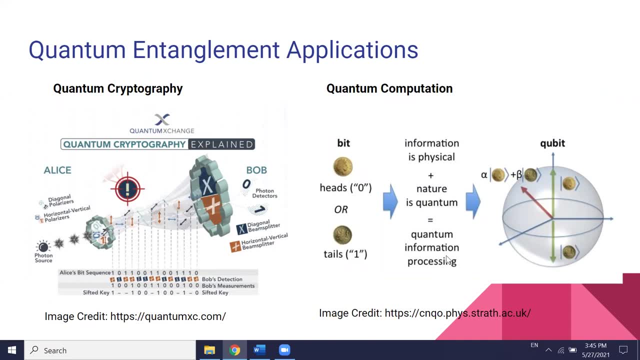 which is called the cosmic hologram by Judy Corbyn. Lastly, I just want to briefly mention about how the topic of quantum entanglement may be significant. Well, the experiments conducted so far show the violation of Bale's inequality theorem, which confirms that a pair of entangled particles 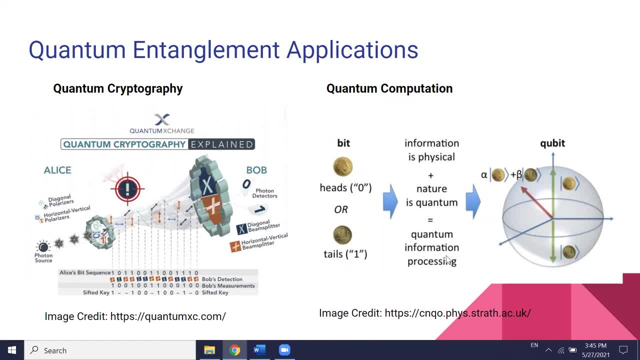 separated by large distance must be considered a single, non-separable object. In other words, it's impossible to assign local realism to each particle separately. Today, quantum entanglement forms a basis of several cutting edge technologies, So here I give you two examples of applications. 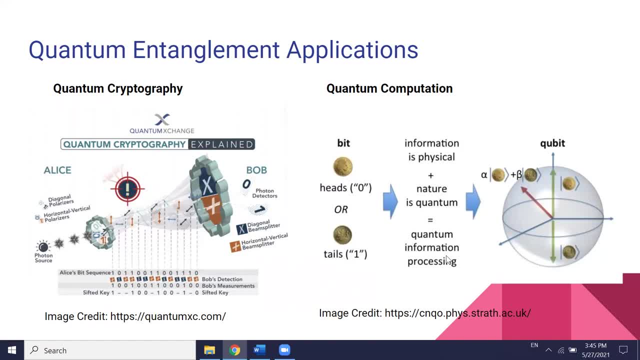 First one is the quantum cryptography. Entangled qubits are used to transmit signals that cannot be intercepted by the third person. I like mathematical encryption. Quantum cryptography uses the principle of quantum mechanics to encrypt data and make it virtually unhackable. And the second application is the quantum computing. 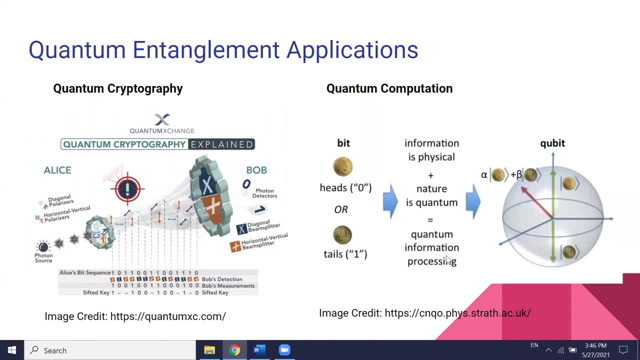 So quantum computing basically, are using the binary values such as one and zero in the superposition, so that the qubits are often measured on either one zero or a combination or a superposition of one and zero. In that sense, quantum computing can greatly enhance.